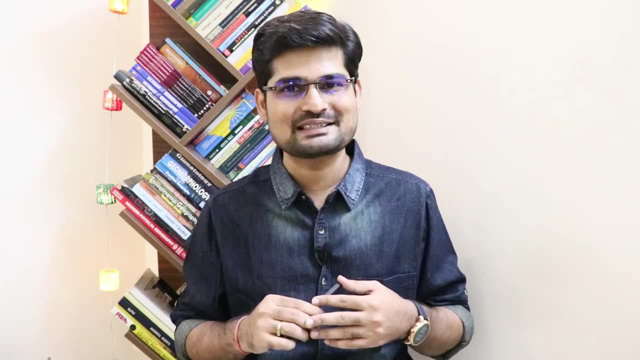 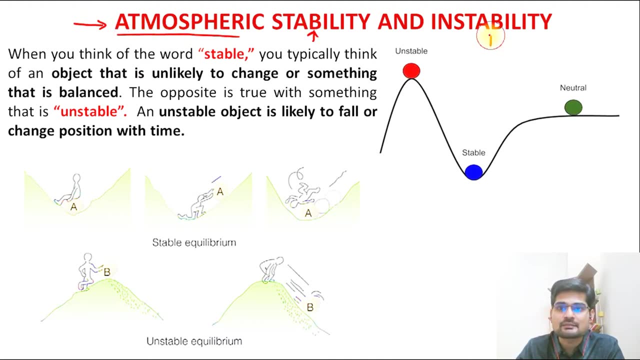 subscribe to our channel and don't forget to share the videos with others as well. So now let's discuss this phenomena that we say atmospheric stability and instability. So the first idea is: what is this? stability and instability? A general connotation of being 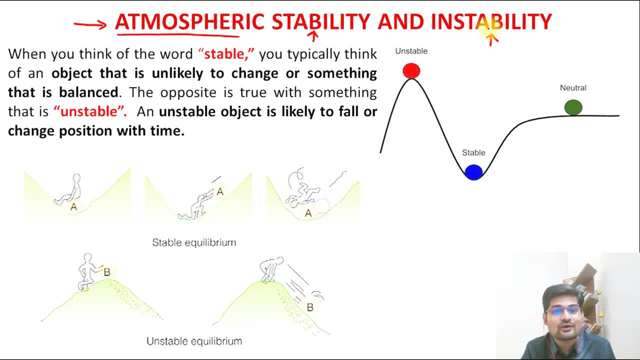 stable is what? Staying at a particular place, just sitting on your chair, being at your place, That is what is stable and what is unstable. When you start moving away from your individual position, that is supposed to be unstable. So remember when we are saying stable and unstable. 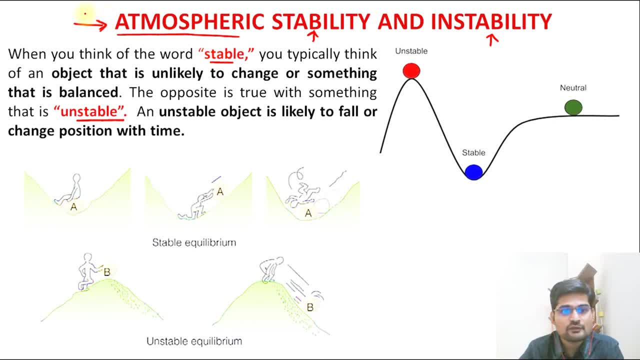 in terms of atmosphere. what are we talking about? So, if you look into these two images here, just see This particular which is sitting on the cliff, this ball- this is highly unstable because with a slight push, slight energy change in terms of, if you say, atmosphere. 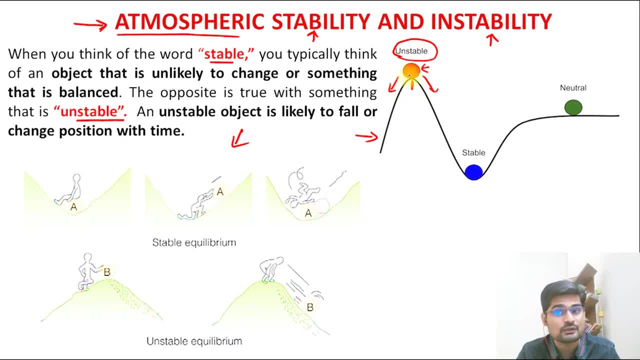 what happens? There is this dislocation and it is highly unstable, But which is here in this valley, if you see this particular location. So if you see this particular zone, it is very stable. It can not go this side. it cannot go this side. it is sitting here at one place. 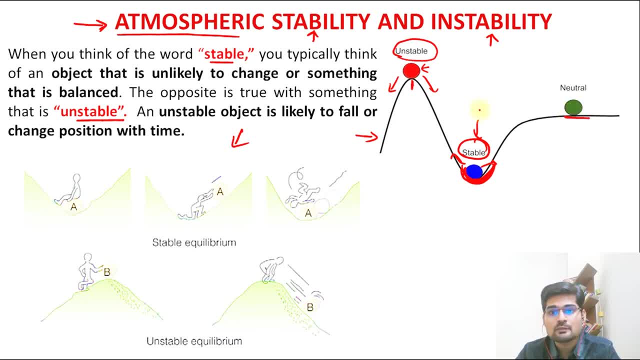 And also third situation. If you see, this is a neutral situation in between somewhere these two. What is this neutral situation? It can either move this way or this way, but even if it moves, it will stay at this particular location itself. It is not going to go anywhere. So that is. 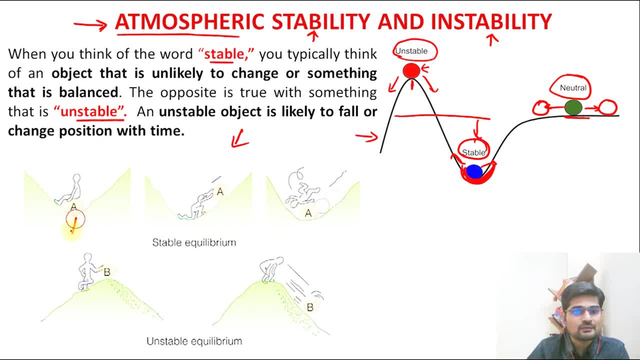 something which is a neutral situation. Similarly, if you observe these images- position A and then position B- what you see this is fairly a stable situation. If you see, even if the boy pushes this ball, it again comes back at the same position. 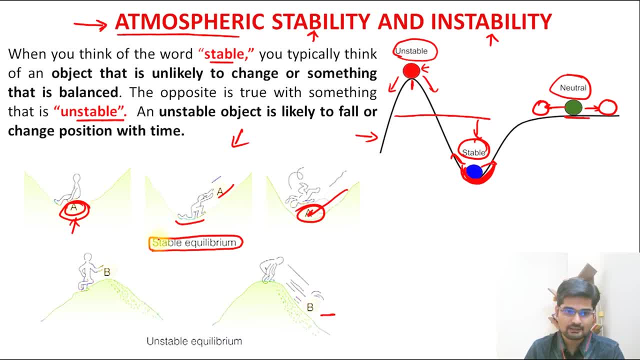 So this is a neutral situation. So this is highly a stable equilibrium position. But what is unstable? If you push it from this particular point, then what happens? It never comes back, So it is highly unstable. So this is what we say is unstable equilibrium. So these are basic concepts about stability. 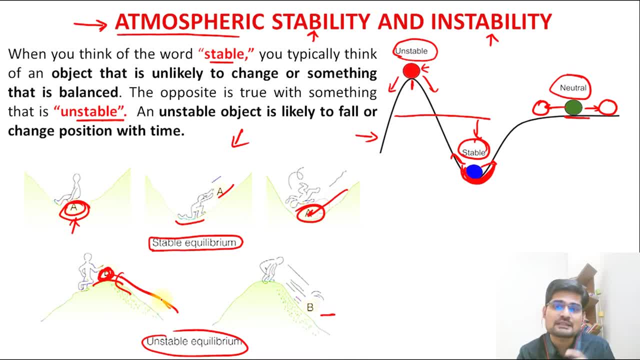 and instability. Let us now understand this concept of stability and instability in context to the atmospheric circulation. Now, for this, it is important to understand two important concepts. The first one is the atmospheric circulation. Now, for this, it is important to understand two important things. One is: what we see is the vertical temperature distribution. 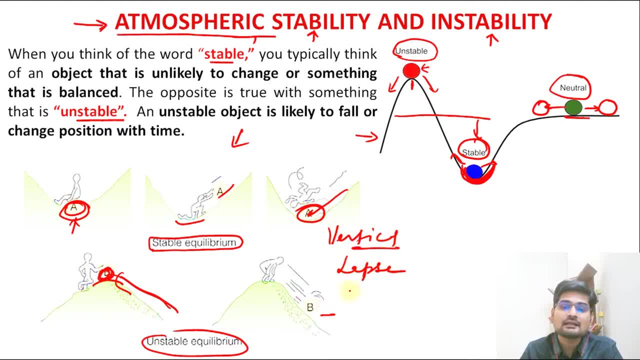 that we have learned in the forms of lapse rate and adiabatic lapse rate. So lapse rate and adiabatic lapse rate tell us about how temperature fluctuates moving ahead in the atmosphere. So inversion of temperature also we have studied. 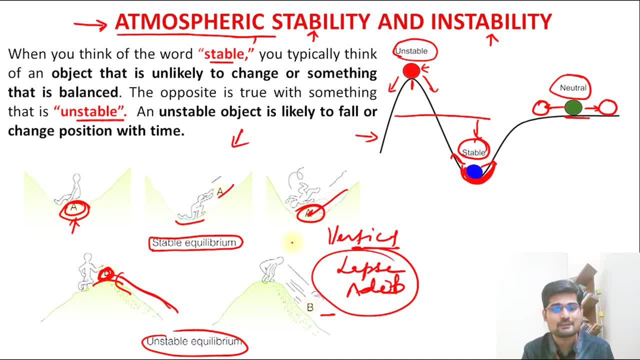 So if you would have not studied about lapse rate and adiabatic lapse rate, it is a request that you please go to the playlist before understanding the stability and instability. Do learn lapse rate and adiabatic lapse rate concepts and details So that it will be. 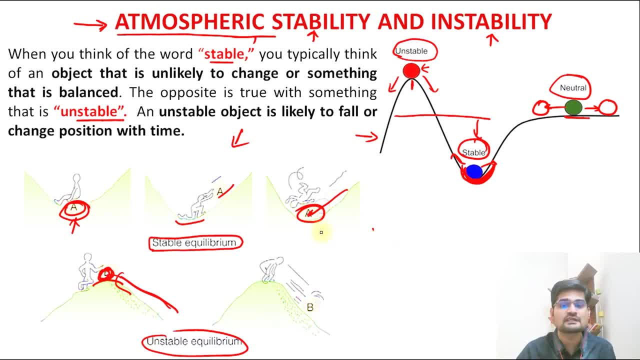 easier for you to understand this stability of atmosphere and instability of atmosphere, as it is directly linked with these lapse rates that we see right, The vertical temperature through elevation when there is a change in the temperature of this air parcel or, for that matter, the entire atmosphere in the troposphere, specifically when we say So. 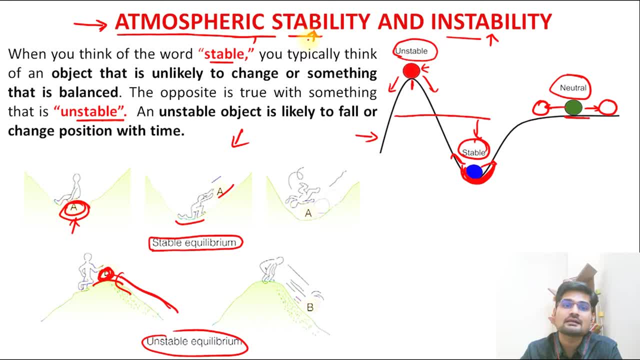 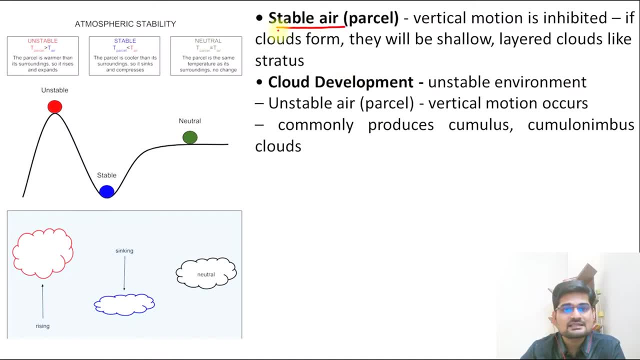 that is important to understand, how stability and instability are linked to this atmospheric. So that is important to understand. So let us now start to understand the two concepts, phenomena. Now let's elaborate further more. So, if we look further more, what do you see? So what is? 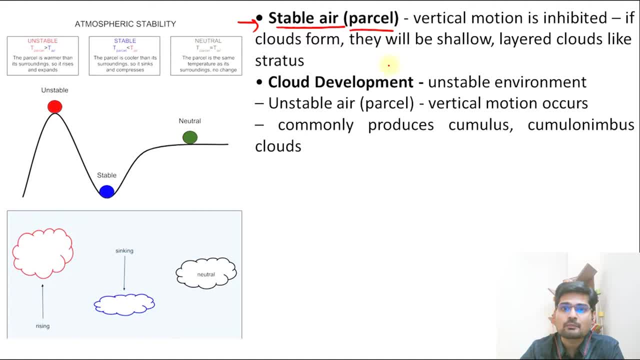 a stable air here. Stable air or a parcel, Parcel is what Remember. it's a packet. So when you order on Amazon and a packet comes, it's like a parcel. It's a fixed entity, right? So if we say: 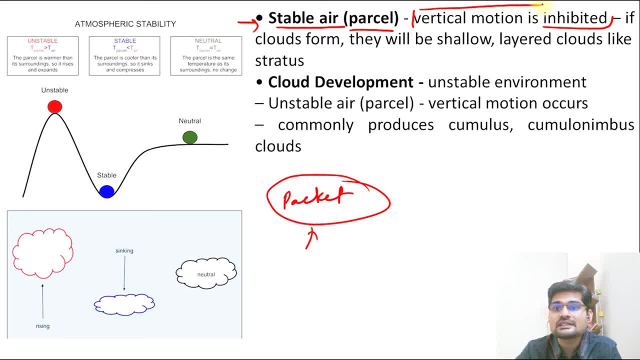 stable air or a parcel of air whose vertical motion is actually inhibited. Vertical motion is inhibited means basically what It is stable: It is not moving upward right, It is at a particular place, right? So this is important. This is where we say it is a stable air parcel. Now, if an air 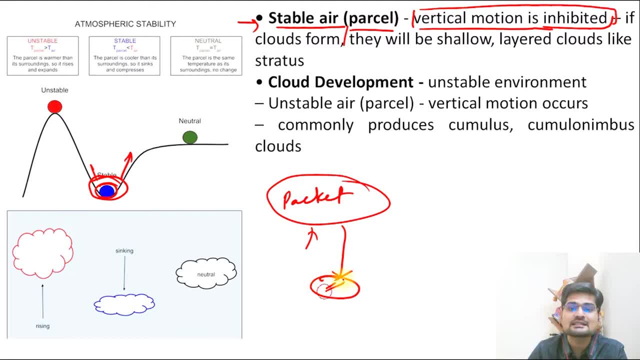 parcel has tendency to actually come down and sit. this is a tendency to actually be stable right, And it is also important for cloud development to be unstable at the same time, Why, If it is not unstable, it will not be rising right, It will sit at the same place. 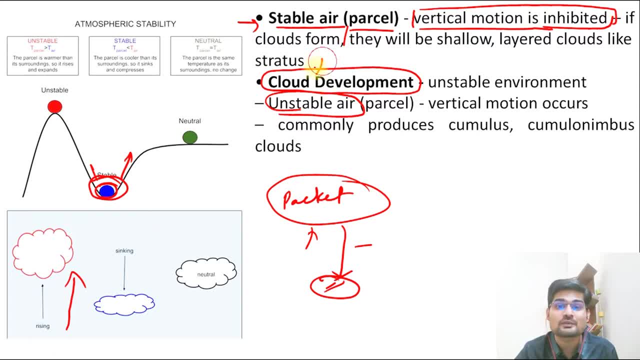 So to rise is important for this cloud formation, right? If the air carrying moisture will not rise, then how is it going to rise? So if it is not rising, then how is it going to rise? So instability is not like something bad for atmosphere. It is important for the cloud. 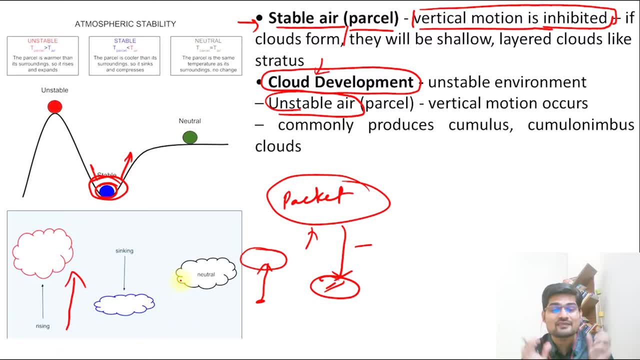 formation. So remember stability and instability when we hear we think like good or bad, It's not like good or bad, It is basically characteristic of this atmospheric circulation. in context, when we see So stability and instability are like yin, yang concept, right, They are actually. 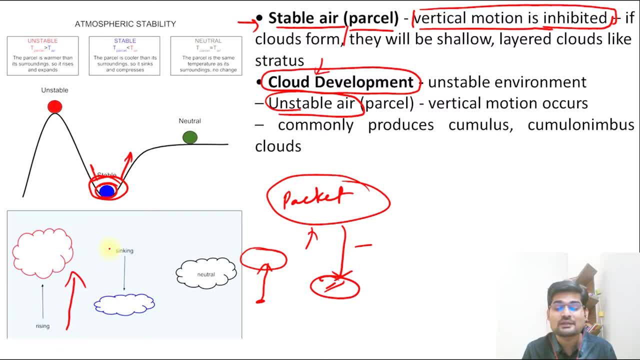 complementary to each other for the entire climatological phenomena, for atmospheric phenomena to operate. So that is why it is important. So, stability and instability, in simple way, is this tendency to actually rise up and fall down. So when you are rising up, you are unstable. you are mobile, you are moving, But when you are 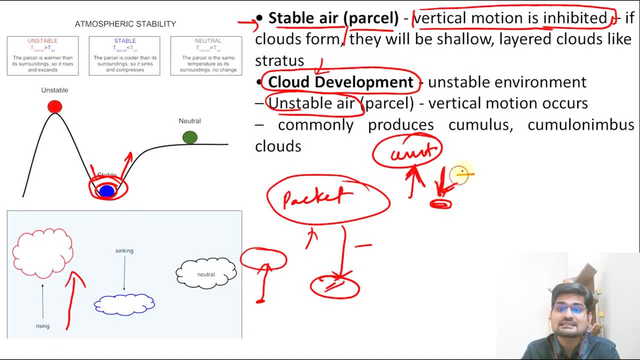 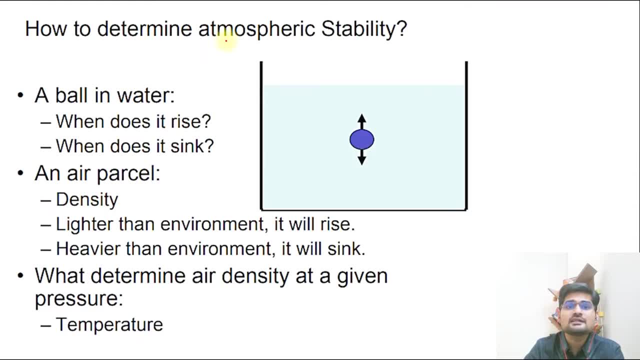 falling down. when you are coming down and sitting at your place, this is a tendency to be stable. That is what the basic connotation is that you should remember. Now, how do we determine this atmospheric stability? So, for determination of this atmospheric stability, what do we do? 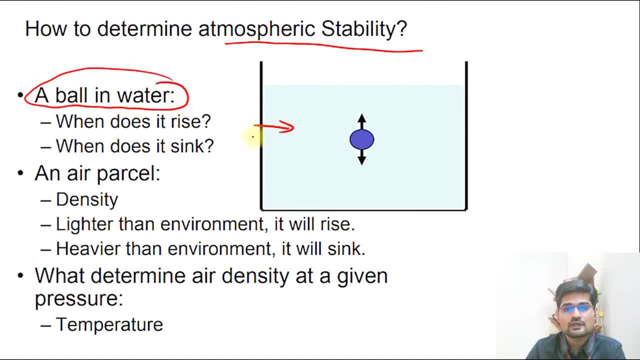 So let's see this example of a ball in water here. What do you see? When this ball is here in water, what happens? When does it rise and when does it sink? Now remember the law of flotation, Archimedes principle, several other. 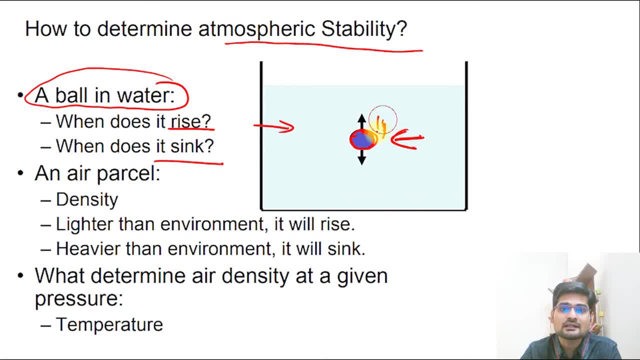 things. So if this mass is actually lighter, it will float up in the air right, And if it is heavier, it will sink down. This is the basic concept, right? So what happens In terms of atmosphere? if you see, if this is a parcel of air, if this is an air packet, what will happen? 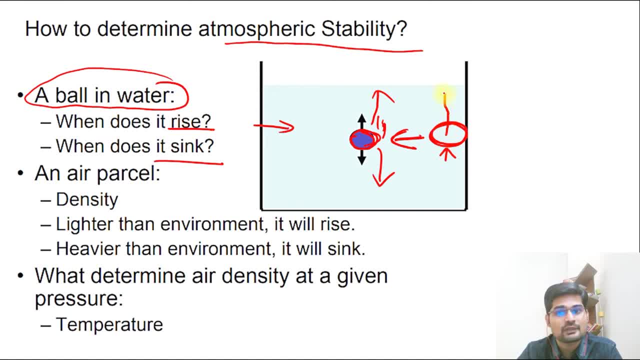 If it is warm, if it is heated, it will rise up, it will float up, But when going up it again cools down. it comes back to the ground right, Because it becomes dense and it becomes heavy. So what happens? Cool air comes down. 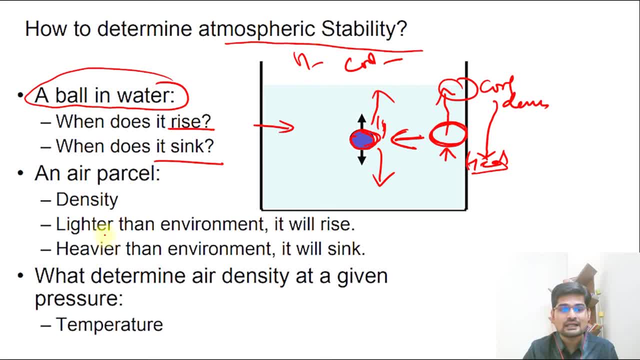 hot air rises up is the basic concept. So the air parcel, what is important here? The density, light, environment- it will rise, heavier than environment it will sink. So remember, when we say lighter than environment and heavier than environment, it means what? 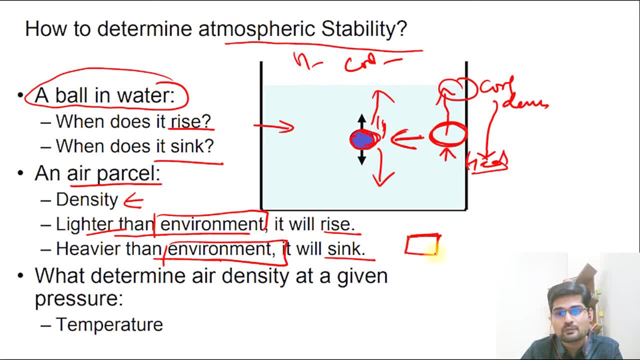 We have already talked about it is a fixed packet. When we say fixed packet or parcel, there is environment all around it, right? So either its temperature will be same or it will be higher, or it will be lower than environment, right? So that is what is, the three different. 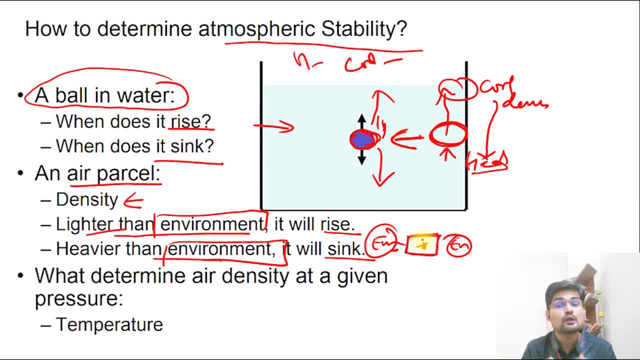 cases. If it is higher than environment, what will happen? If it is lower than environment, what will happen? If it is same to same as environment, what will happen? So this is what is all dependent upon this factor: that atmospheric stability will be there, or 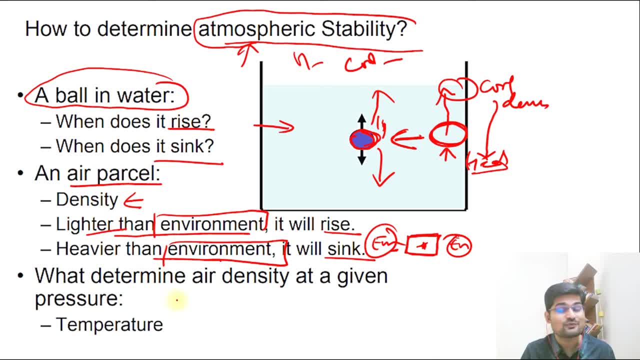 instability will be there. So the major driving force again: what is the major driving force behind the stability and instability? It is the temperature, right, So this is important- right, At a given pressure, how much is the temperature? So if temperature is injected in an air parcel, 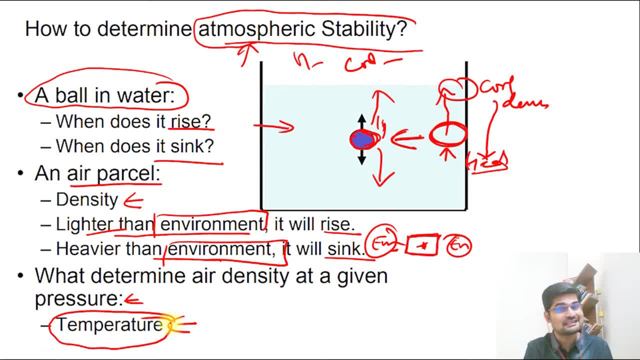 what will happen? The molecules will expand, right, The volume will increase. it will go up as it becomes light. So as it goes up, it will start to increase in the volume as well. So this is what the entire phenomena happens on the earth. So this is what the entire phenomena happens on the earth. 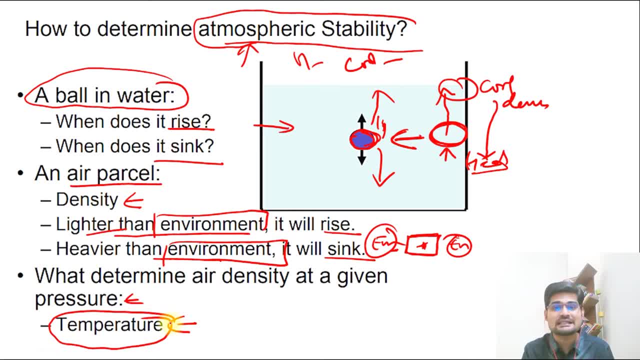 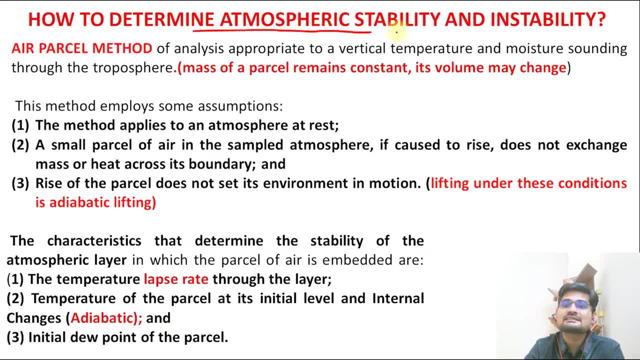 So this is what the entire phenomena happens on the earth. So let's understand this stability and instability in details now, So experimentally, how do we determine this atmospheric stability and instability? A very common method. you must have heard through several lectures of others. 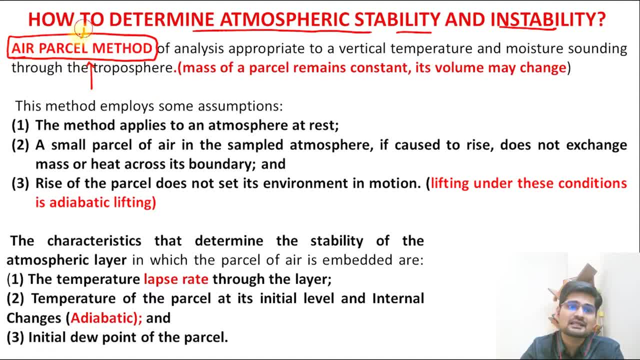 many people, many scientists, many teachers have taught you the same method, that is, air parcel method. Now, why is this air parcel method so famous? Why everybody talks about it? The first important thing is that we need to understand a phenomenon which is natural. So unless we are able to actually experimentally understand the 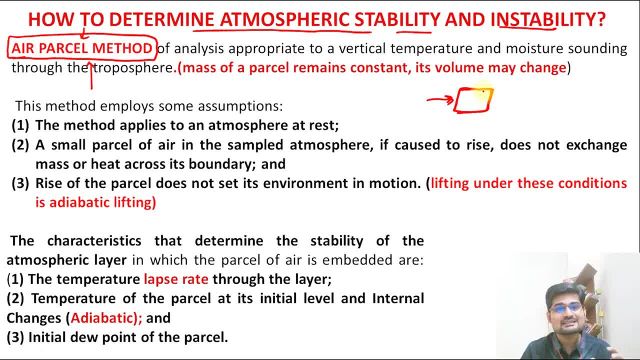 process. we cannot actually generalize it. So this is a scientific kind of study where what we do is we take a fixed unit volume of air right, That is a parcel whose mass is constant right, And what is expanding? The volume is changing. Why volume is changing? Remember the gas loss Because of the 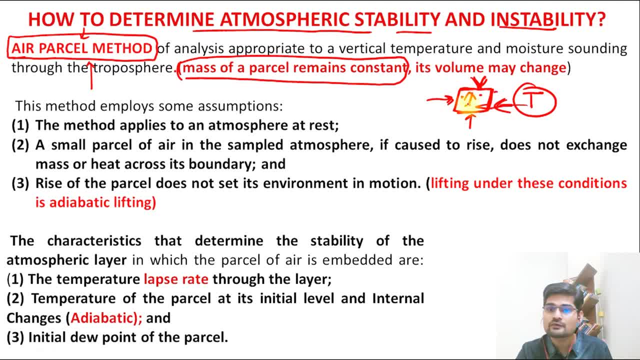 temperature changes right. So if temperature changes, what will happen? Molecules will go away from each other, So volume will expand. If it is cooling down, molecules will come back. condense, it will become denser, it will fall down. This is the entire mechanism. But this air. 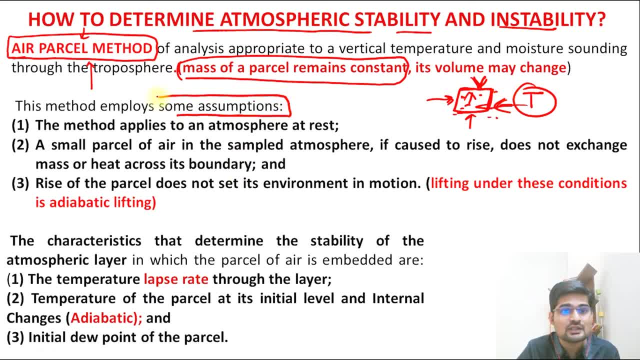 parcel method has some assumption. Now, this is something unique that you need to understand that this is not discussed generally when people say air parcel method. So what are the assumptions? Remember, the method applies to atmosphere at rest. So it is considered that when this parcel 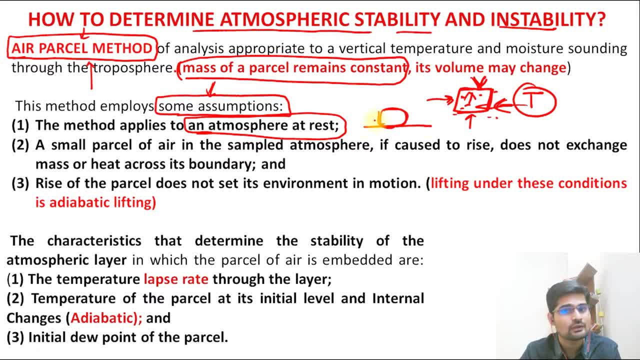 is at rest, it is not moving, it is just fixed here. it is sitting on the ground is the first assumption, right. Then small parcel of air in the sample atmosphere is caused to rise. Now this is just a single important sample part of the atmosphere, So it is kind of a sample. 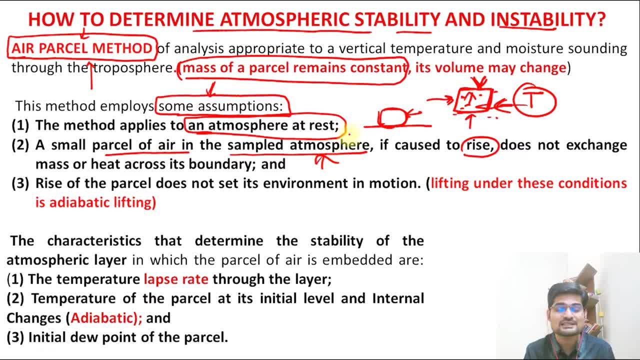 Remember, in scientific studies we take sample, we apply method to the sample, then apply that important result on the general atmosphere. So this is how this resultant is happening here also. So we take a sample air which is called air parcel right Now. the rise of the parcel does 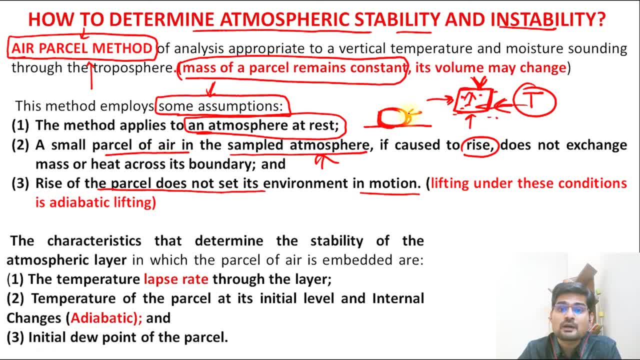 not set its environment in motion. Now, remember, the rise of this parcel does not set its environment in motion. this environment has nothing to do, it is not affected by this rise. So that's why we just take this parcel and see the impact of what happens with this temperature and volume changes on this. 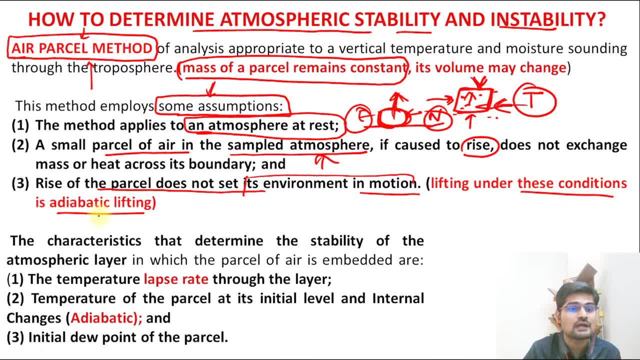 air parcel. So lifting under these conditions is supposed to be through adiabatic process. So that is what the pressure, temperature changes are important. volume changes are important where one factor is constant. The characteristics that determine this stability of the atmosphere are what? 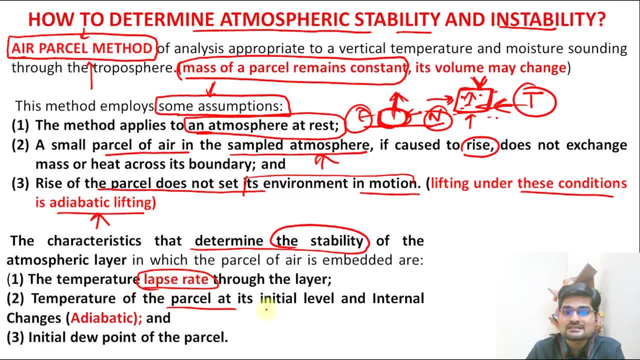 The temperature lapse rate through the layer, then temperature of the parcel at initial level and internal changes that happen, that is, internal changes happen that we study as latent heat of condensation, dry and wet conditions of adiabatic process in the thermodynamics. 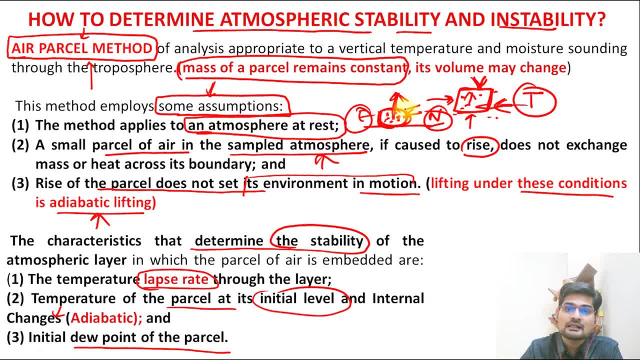 So initial dew point of the parcel. now remember this parcel has initial dew point. that is important where the saturation happens, where the cloud formation happens, where the latent heat release happens. So these are the important points to remember. So when you are writing an answer on stability and instability, don't just start mentioning 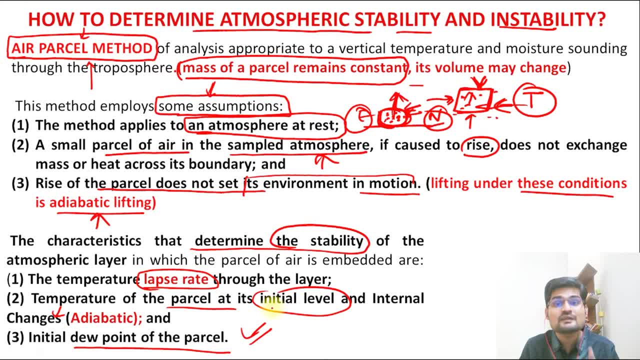 air parcel and start with lapse rate and adiabatic lapse rate. Always mention these points. that will make your answer look good, because you know the assumptions behind this parcel method of actually determining the atmospheric stability and instability. So what are the golden rules? 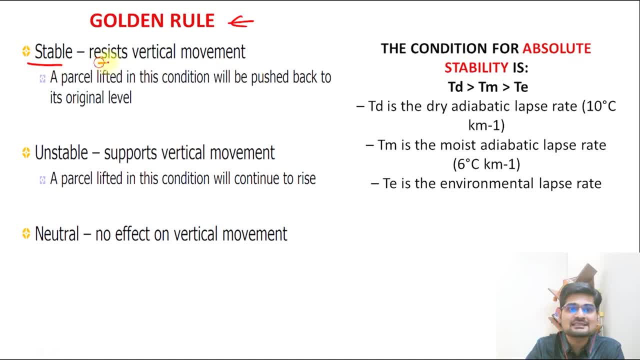 Now remember, golden rule is the first one. stable means resists vertical movement. right A parcel lifted in this condition will be pushed back to the original level. So even if we take it to this particular height, it will again come back. or even if it is this: 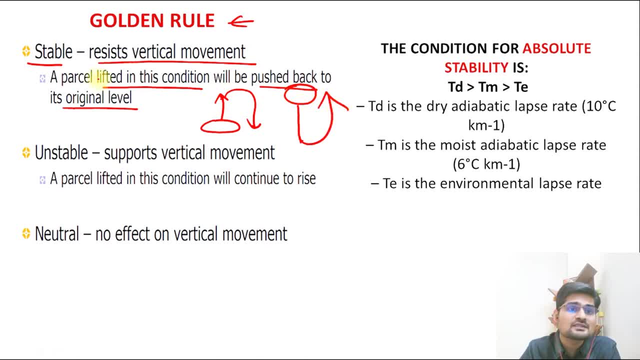 height we throw it down, it will again go back to the same because of this stability condition that we see right, Because of the temperature changes that we observe. So, in stable situation, unstable situation, it means that it has a tendency to actually 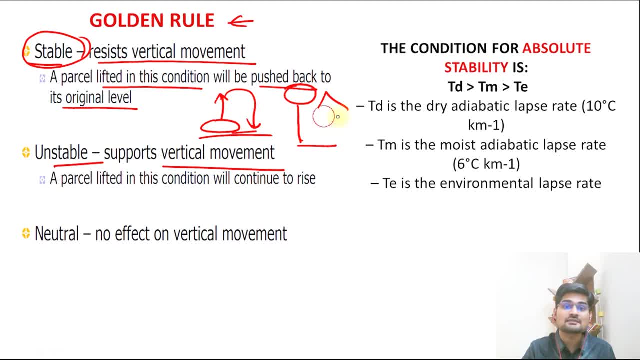 rise, that is, vertical movement is involved here. So that is why it is important that vertical movement tendency is triggered by what Is triggered by heat action, by insulation action. right, That is important, But neutral is no effect on vertical movement. So that is another third case. 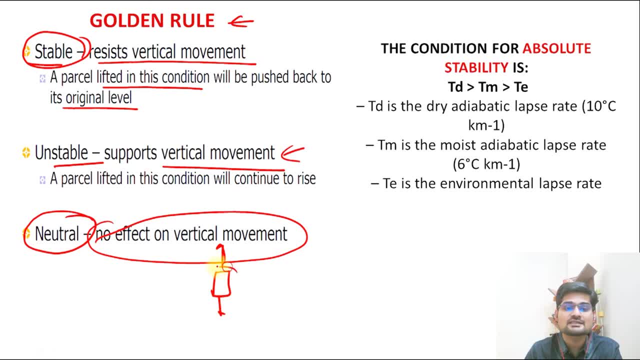 If this air parcel has no effect of moving up or down, it is just fixed in this particular state, where environmental temperature and parcels temperature are equivalent, then this is a neutral state. So conditions for absolute stability is here. Remember, Remember what it is: dry adiabatic lapse rate, which is normally 10 degrees C. it is assumed 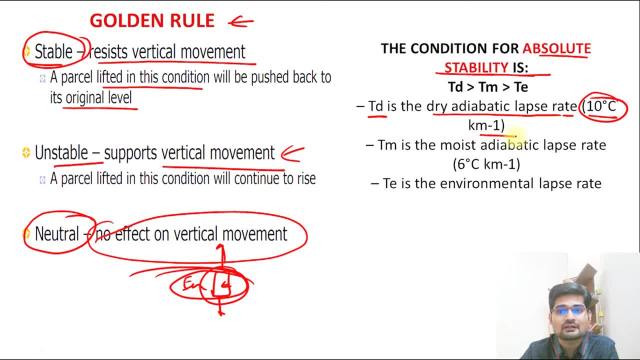 as an average value. So this is 10 degrees C per kilometer. This is called dry adiabatic lapse rate, which is Td here. so Td which is greater than Tm. So Tm is what Moist adiabatic lapse rate, which is average as 5 degrees somewhere or 6 degrees per kilometer. 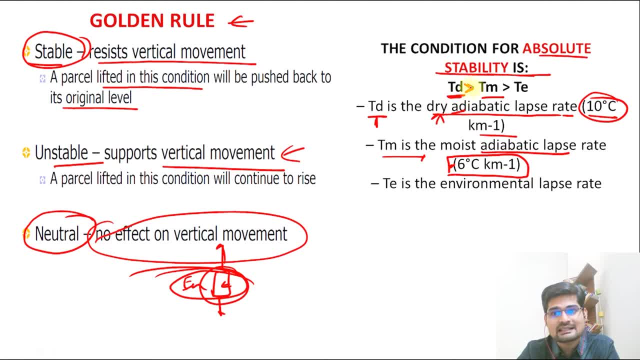 So remember, this is the Tm, So Td is greater. dry is greater than Tm, which is further greater than Te, which is the environmental lapse rate. It is called Elr If this is the situation where dry adiabatic lapse rate is most effective, factor which 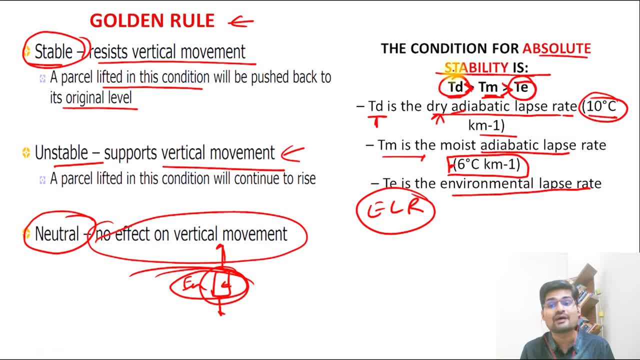 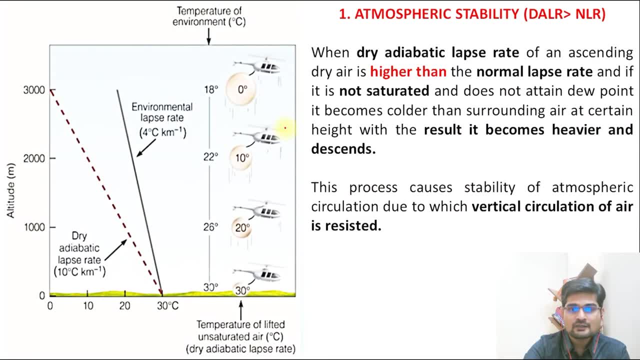 is most dominating factor, then moist and then environmental lapse rate. it means it is absolutely stable condition. There is no tendency of the air to actually go ahead. So what you observe here is this atmospheric stability. Now there is a case, Dalr. 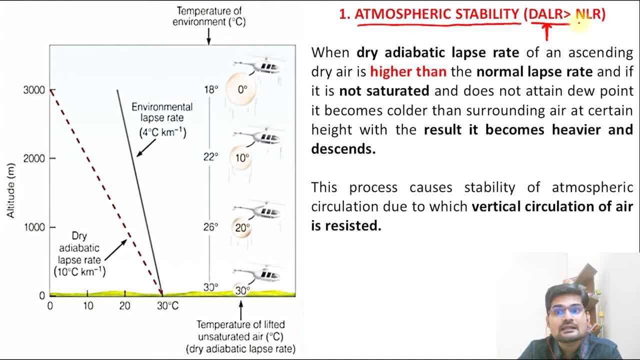 What is this? Dry adiabatic lapse rate? It is greater than normal lapse rate. So, if you understand this situation, what is happening? dry adiabatic lapse rate is higher and normal lapse rate, or environmental lapse rate, is lower. 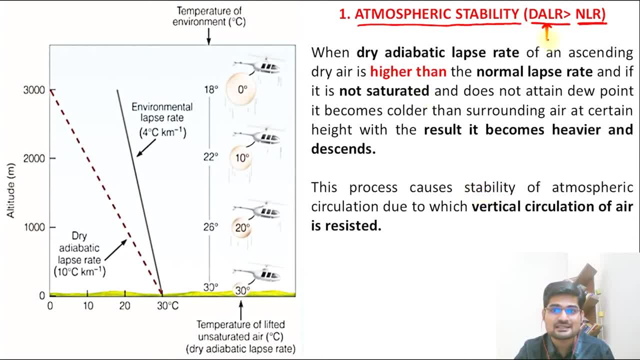 In this case, what happens if it is not saturated air? remember it is dry air, it is not saturated. So what will happen? It does not attain dew point and it becomes colder than surrounding air at a certain height. With result, it becomes heavier and decent. 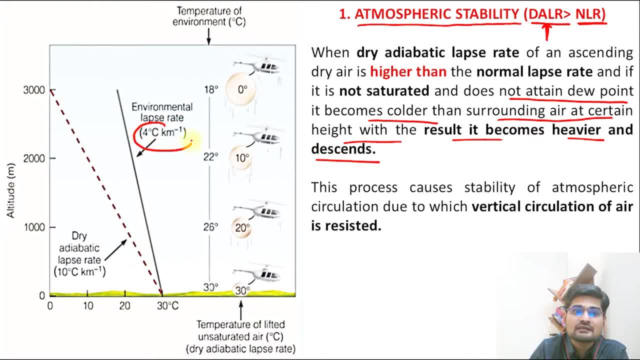 So remember, as we discussed what happens here, this is roughly environmental lapse rate. It is 4 degree right. And what is here? Dry adiabatic lapse rate is 10 degrees, So it is greater. So what do you observe here? 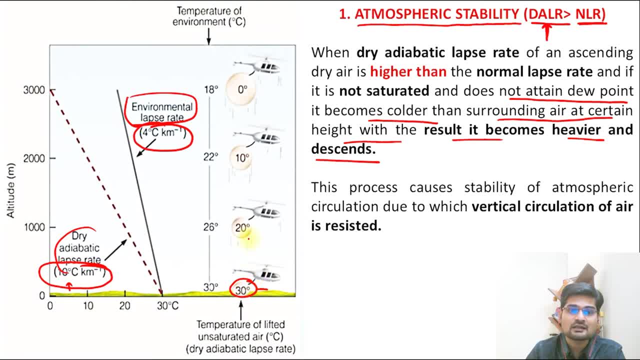 What is happening? Remember this particular parcel of air is 30 here, It is 20 here, It is 10 here, It is 0 here, But environmental lapse rate is lesser. So what happens? It is 30 here. 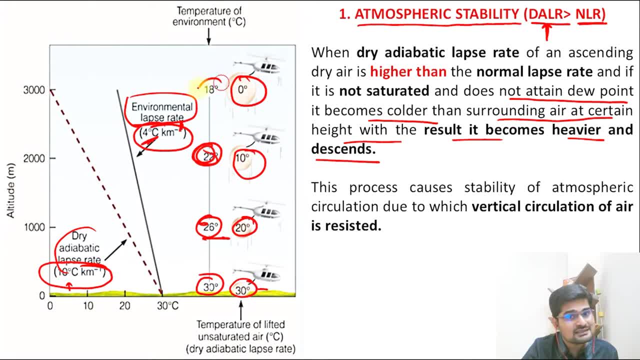 At the same height, it is 26.. At the same height, it is 22.. At the same height, it is 18.. So what will happen If this layer temperature is 18. And if this parcel temperature is 18.? 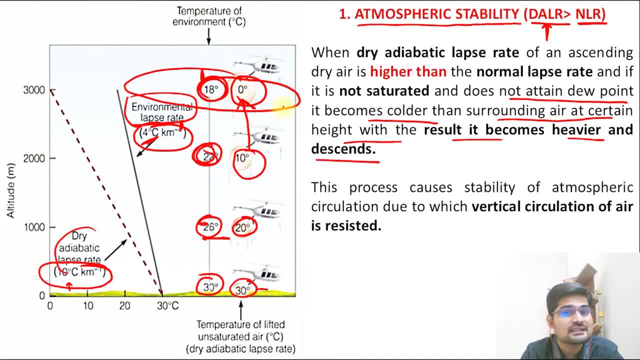 So what will happen If this temperature is 0,. just understand what is the situation here. What will happen? This heavier air will starts to descend down. This cooler air is heavier, So it will starts coming back right. It will not go further more. 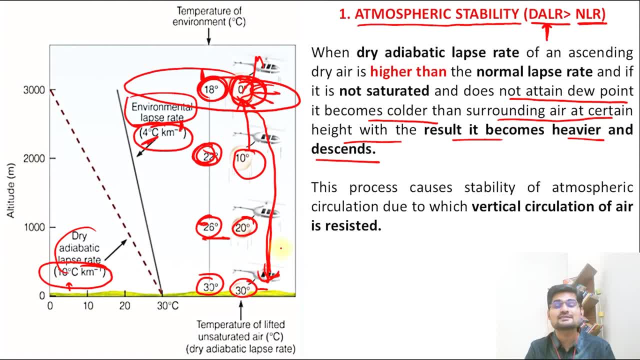 So it will have a tendency to come back, And that is where it is important to understand when this tendency to come back is there. what is the situation? It is a stable situation, right? This is how the difference of this DALR. 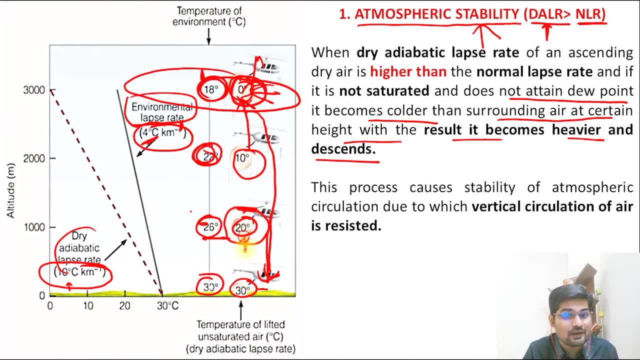 That is dry adiabatic lapse rate Right, The dry adiabatic lapse rate of this air parcel and the environmental lapse rate or normal lapse rate situation is actually attached. So DALR is greater than normal lapse rate or environmental lapse rate. 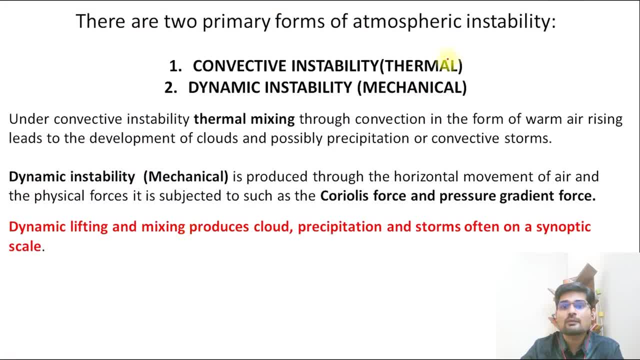 A stable situation is expected Right Now. further, if we talk about atmospheric instability, which is where we are more concerned, because this is regulating the entire climatological phenomena, that is why instability is very important, So it has two types. 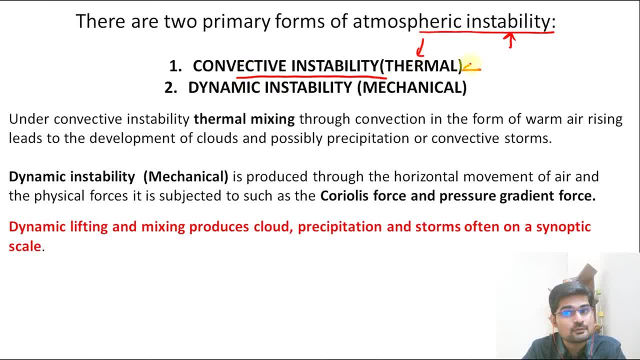 One is called convective instability. that is thermal, that is heat based, So convection happens right from low to high and again come back. So this is what convective cycle looks like. So it happens like that. Then we have a dynamic instability which is of mechanical nature. 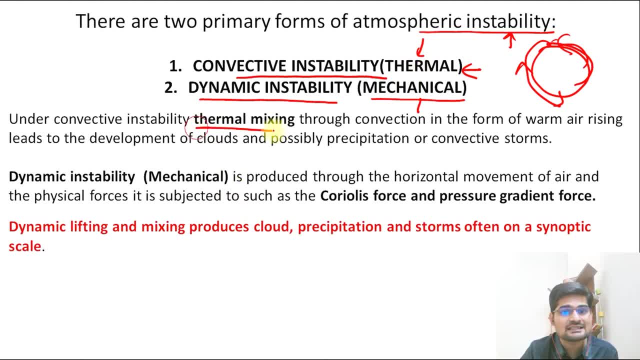 So let us understand convective instability, that is, thermal mixing of hot and cold air that we know. But dynamic instability is mechanical in nature. It is produced through horizontal movement of air and remember Coriolis, force and pressure gradients. These are the forces that are important for this dynamic instability. 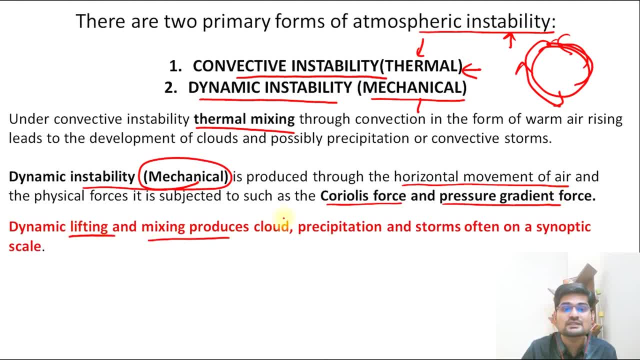 Right. These are the forces that are important. So dynamic lifting and mixing produces cloud precipitation and storms, often where on a synoptic scale, on a regional, greater level. that is important to understand here. So convective instability is the major part of atmospheric instability that we are talking. 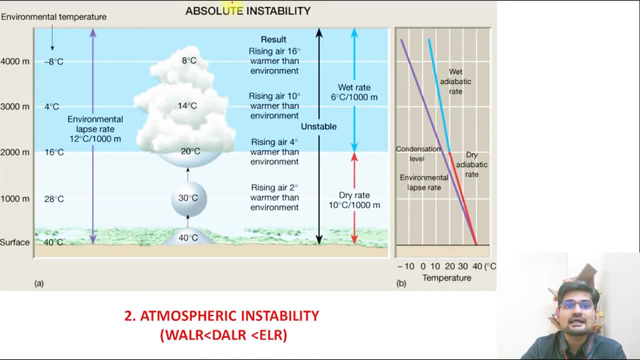 here. That is, the thermal instability. So now let's understand what is the case of this absolute instability. When does this absolute instability happen? So simple way to understand is when wet, adiabatically Wet adiabatic lapse rate is smaller than dry adiabatic lapse rate, which is smaller than 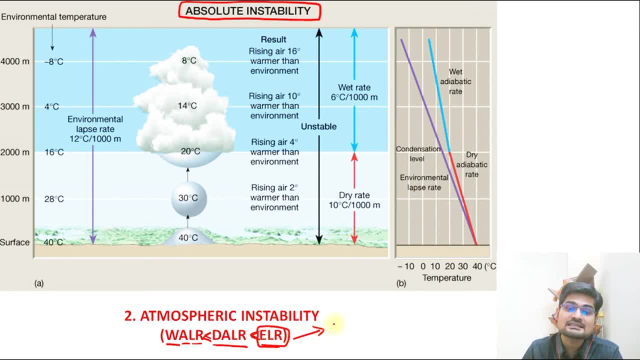 ELR, environmental lapse rate. It means ELR is the greatest when environmental lapse rate that we say as normal lapse rate, suppose its value goes very high, then what happens? Let's look at this particular situation Now. remember: this is that parcel of air right. 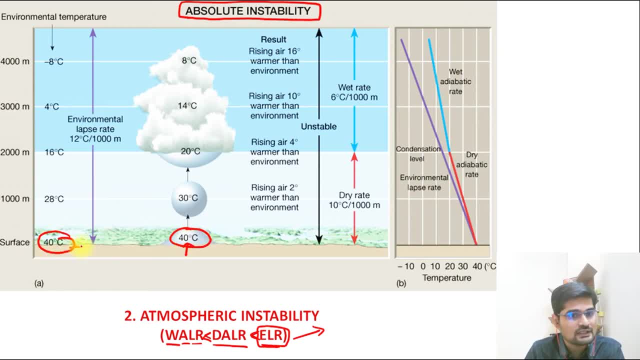 It is at 40 degrees C and the normal situation is also on the ground environment is 40 degrees. So these are the forces, So these are both at the same temperature. Now it is important to understand what is the role of this environmental lapse rate. 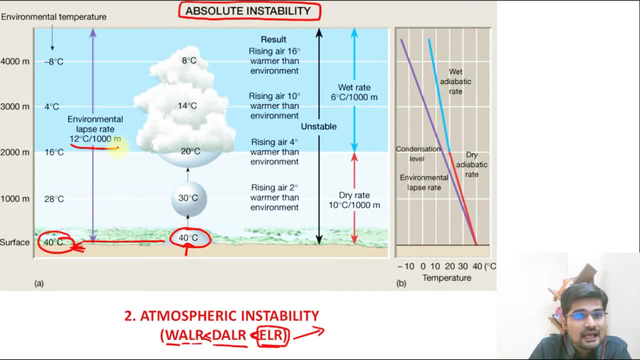 and the other lapse rates. So here what you see is environmental lapse rate is this value, that is about 12 degrees C. So for every kilometer there is a 12 degrees C reduction. right, But at the same time, what is in the wet situation? 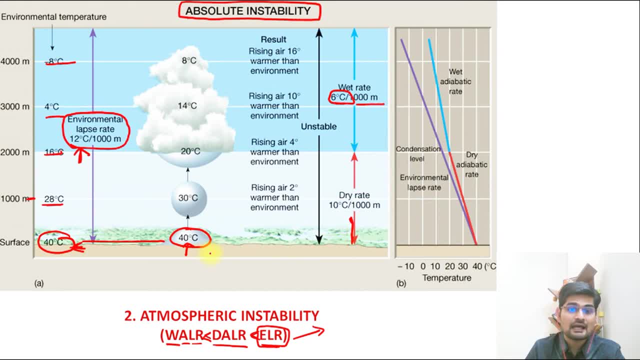 It is 6 degrees C for every kilometer. right, And what is the situation of this parcel of air? It is again the 10 degrees C, Because it is 10 degrees C. So what is the wet situation? It is 6 degrees C for every kilometer. 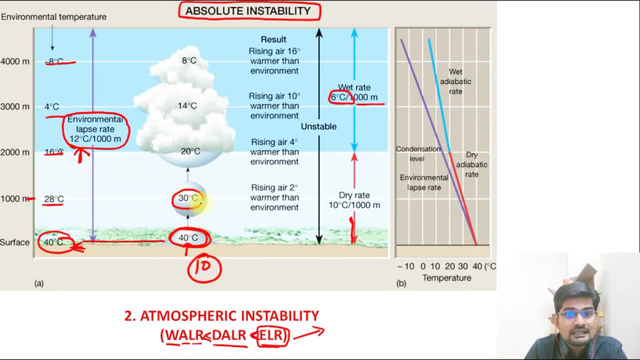 It is dry adiabatic lapse rate. So where it is 30 in the same layer, it is 28 in the normal condition. that is environmental condition. right, Where it is 20, it is just 16.. So what is the situation here? 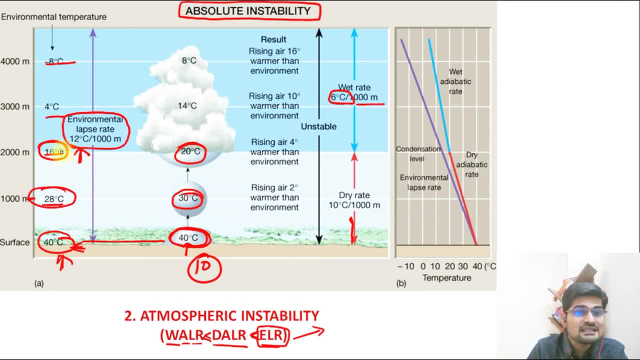 Can you see, Can you observe the situation? What is happening here, On the same layer? what is happening? The atmosphere condition, the normal environmental condition, is actually lower and this parcel of air is actually greater. So what will happen? What will be the tendency of this parcel? 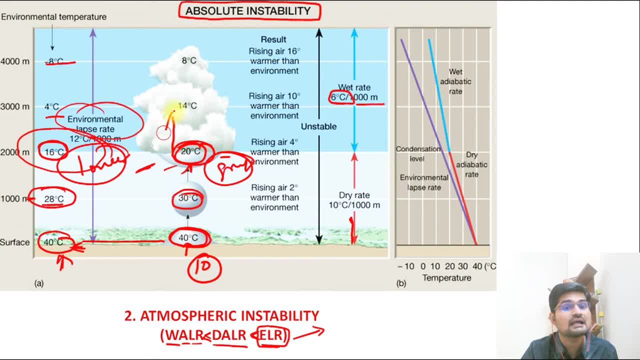 Remember, it is still greater than the normal. It means it will go further ahead. right Then what you see, 4 degree, 14 degree. It will go further ahead. So this is the tendency of going ahead, ahead, ahead and ahead. 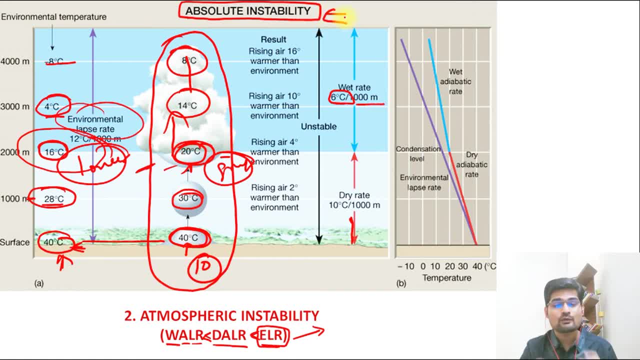 This is what the tendency is about: absolute instability. and why this happens? Because of the change of Elr, respective changes of temperature. if the environmental temperature layer is more, then what will happen? And if the environmental temperature in the layer is less, then what will happen? So these are the two cases, So remember what is here. This ELR is the greatest. 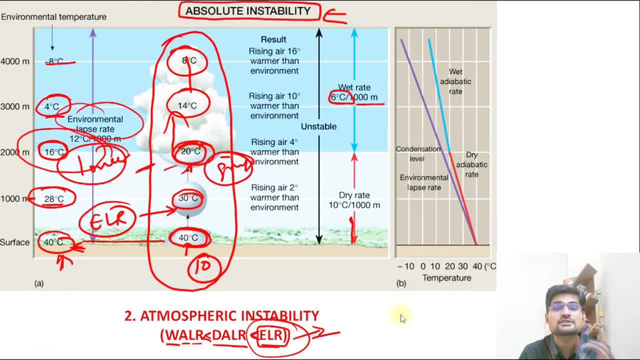 right. So when it is the greatest, then absolute instability. So remember, when you see that environmental lapse rate or normal lapse rate is actually increasing, it means there is high convective situation happening. So that happens in extreme summers that we observe right Now. the 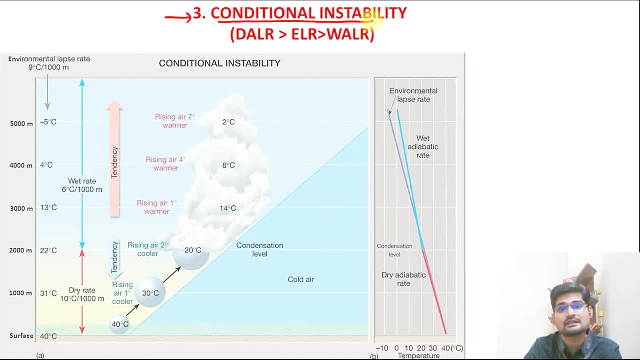 next condition, or the third condition, is a conditional instability. Now this is very interesting. Normally in ELR situation, that is normal environmental lapse rate. we understand how the situation operates. When ELR is greatest, it becomes very unstable. When ELR is smallest, it is a stable situation. So now let us look here. What is the environmental lapse rate? It is 9. 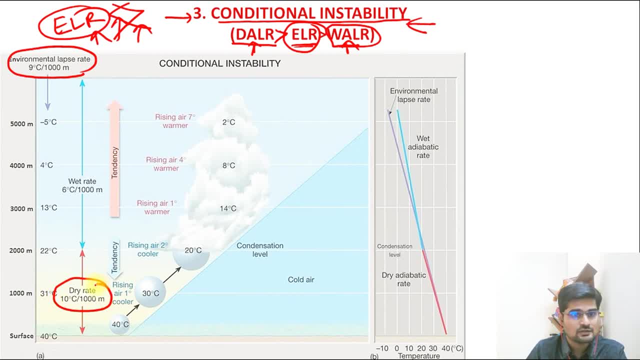 degree. What is the dry adiabatic lapse rate? 10 degree, So this is greater, Dry is greater, But wet is actually 6 degree. So this environmental lapse rate is falling in between this, Remember, 9 is the ELR and DALR is 10. 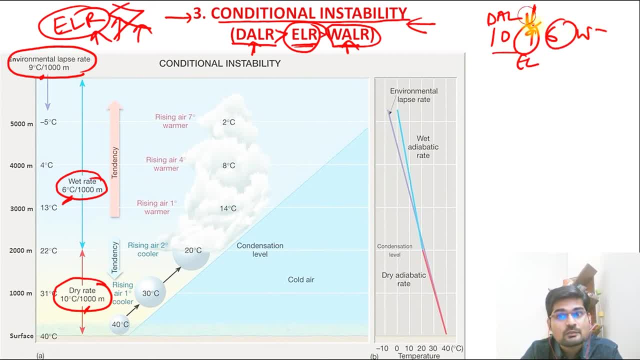 and WALR is 6. So it is falling in between. So, in this situation, what will happen After a particular altitude? Now, this is interesting here- that after this, 40 degree goes, 30 degree goes 20 degree. This is a level where it reaches a dew point. Remember why? Because 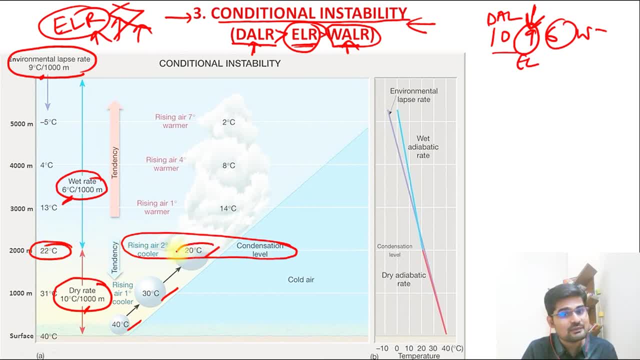 it is 22 degree C. What is the change here? It is 22 degree C while at the same time it is 20 degree C, So it means ELR is now greater here in this layer, and this is cooler. It reaches dew point, So when 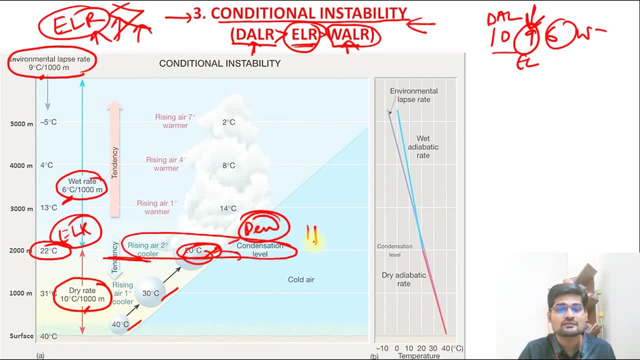 it reaches dew point, there is a change. that is because of the latent heat, Remember. so latent heat is released of the condensation, cloud formation, rainfall happens. But after this latent heat is added, still, the temperature goes up. Why? Because of this water. So the temperature, 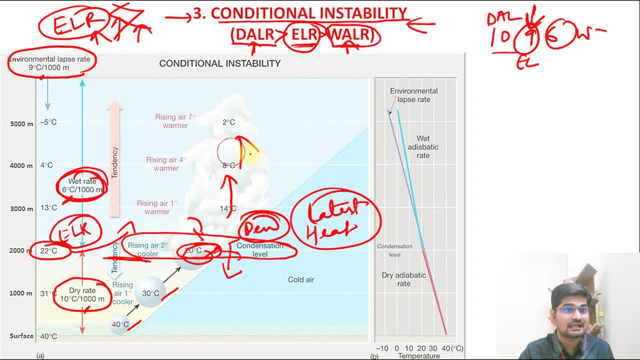 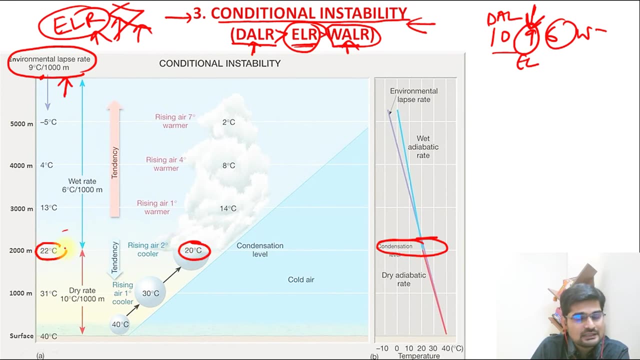 goes up. So wet adiabatic lapse rate. it goes ahead and further ahead. So this is where it crosses the limit. So what we observe here is that, till a particular point, which is a condensation level, till this point, what do you observe? This is 20, right, and this is 22 degree, right. So what is this? layers? 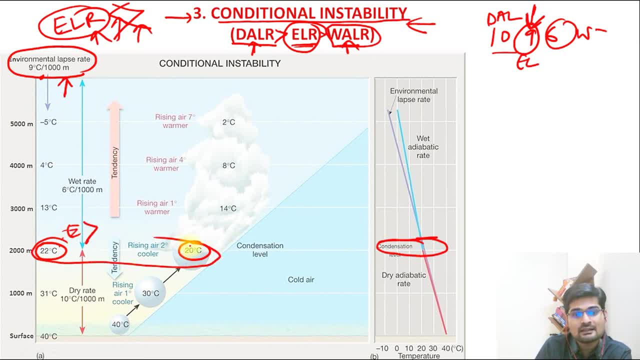 property. here, ELR is actually greater than DALR till this level. But once this latent heat is added, what happens? This latent heat is added, This latent heat is added, This particular latent heat does a change. and that is where, in the next segment, what happens. 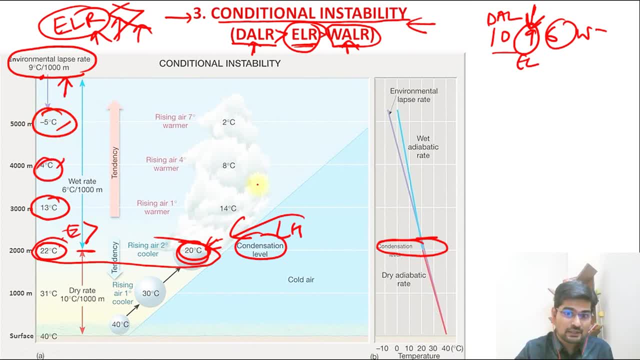 This is 13,, 4 and 5. That is minus 5. But here the temperature has been added So it is greater now. So this is where there is a change. It's shift. It means what you observe is due to this wet. 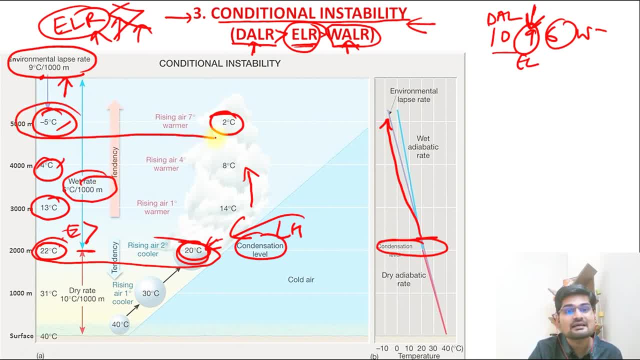 adiabatic lapse rate. there is again a change in this layer and what you see? The warming is there in this parcel of air, and if it is warming, it will go ahead right. So this is what is again an unstable condition, or instable condition, But till a. 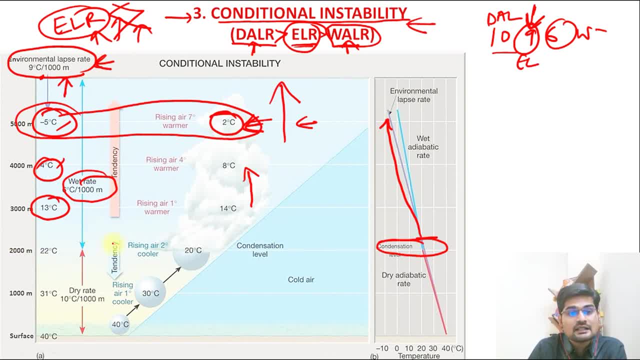 particular extent it was stable. So what you observe is, till a particular extent, that is, till this particular height, when environmental condition is actually warmer and this is cooler, then it has a tendency to fall down, But after this it has a tendency to pick up. 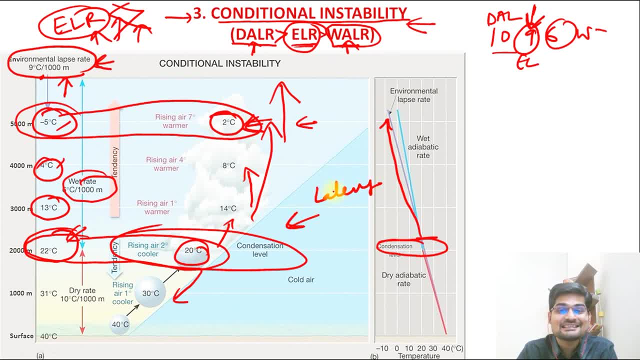 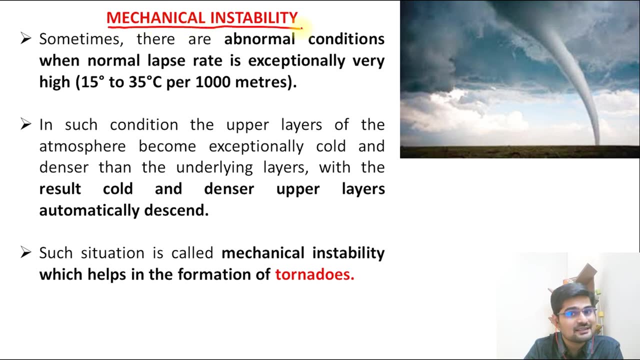 This condition is actually driven by what? Latent heat. So latent heat is part of this wet adiabatic lapse rate, and that is what changes the equation. That is why it is called conditional instability. Now, the last part that we need to discuss is this: mechanical instability. Now remember what happens sometimes due to atmospheric anomalies, abnormal conditions, The normal lapse rate goes to high, to extreme right, Almost like 35 degrees C. So suppose if normal lapse rate goes extremely high, what will happen With each kilometer there will be a major change in the temperature, major reduction in the temperature. 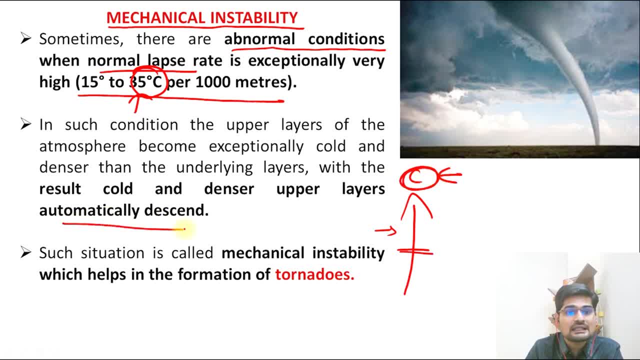 So at upper atmosphere there will be what happening Automatically? a cold situation created because of this high change in or high reduction. So upper atmosphere becomes extremely cold. So if it becomes extremely cold, what is the tendency? It becomes cold, it means it becomes dense and it has a tendency to fall down very quickly as it becomes very cold quickly. So when 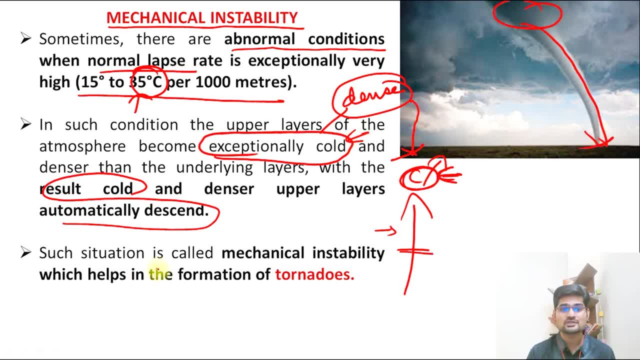 it fall down very quickly. thing happened. what is the situation here? It is a mechanical instability. It pushes the air down and that is where this tornado is formed. That is where mechanical instability is important, right? So that is what we understand by the atmospheric stability and 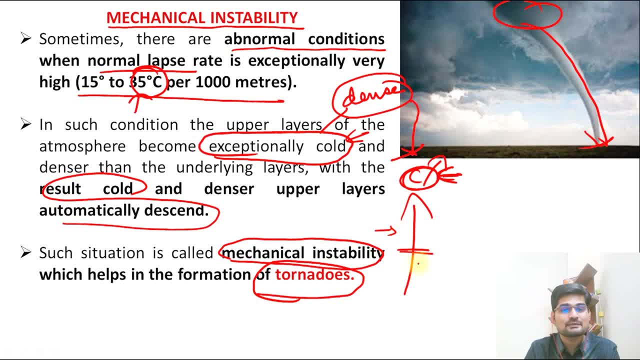 instability. So I hope you understood the stability part and instability part of the atmosphere in a clear manner. So stability is when the tendency is to actually subside down this air and it will only depend upon what is the situation of environment and what is the situation of this. 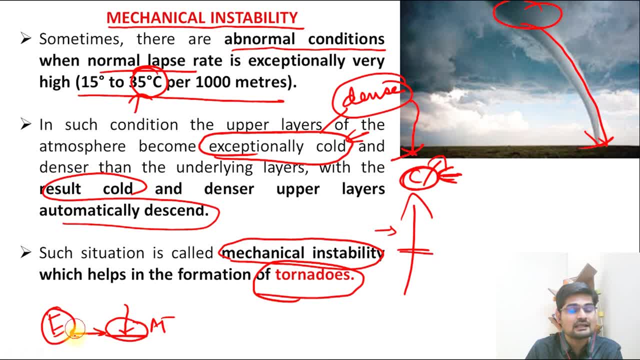 parcel of air. If there are temperatures are in a very low temperature, then there is a tendency to subside down. Now there is a tendency to subside down. So if there are, temperatures are in a very low, varying in what ways they are varying. that is where the stability and 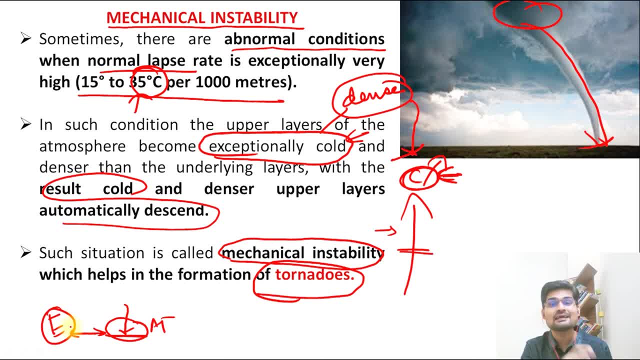 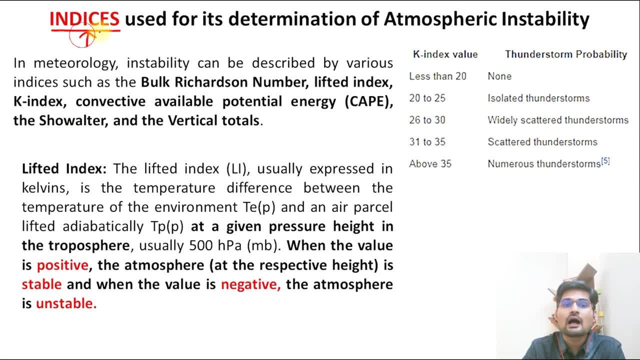 instability. we have to learn, in case of normal lapse rate and dry and wet conditions, of adiabatic lapse rate and at last, we also need to learn about this fact that how do we measure this? so, to measure this, there are certain indices which have been created. for example, if you see bulk Richards and number lifted, 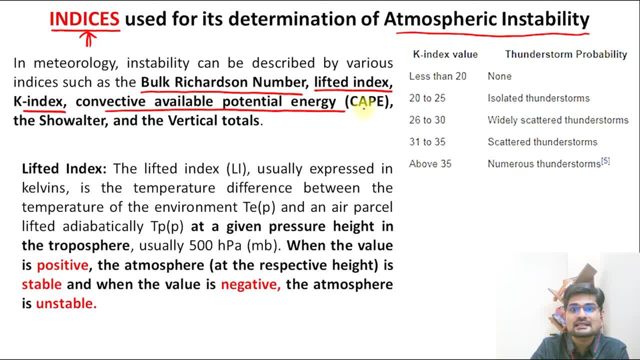 index K index convective available potential energy. that is called Cape and shorter than vertical totals. all these things you just remember the names at least. don't go into the details, but these are important indices that are used to actually determine or measure the atmospheric instability you can. 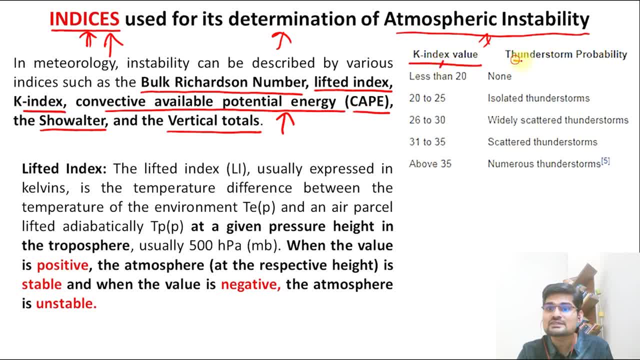 pause the video and see for yourself how this key index actually denotes the thunderstorm probability. so the value and associated thunderstorm probability is here. then lifted index is something which is also very interesting. so when lifted index is positive, it means a stable atmosphere. if lifted index is, 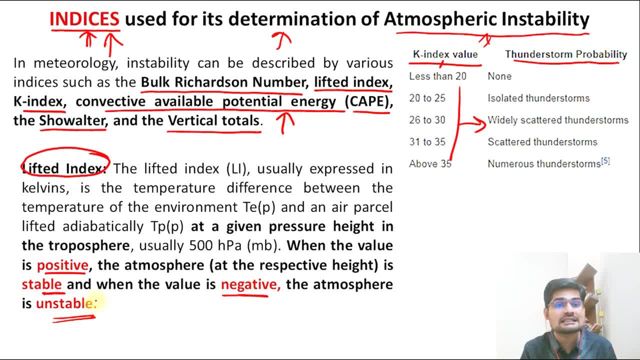 negative means an unstable atmosphere. So these are important indices. So this is what you need to also remember, along with the conditional situation of instability: Instability depending upon the lapse rate and the adiabatic lapse rate of dry and wet condition. So remember this. 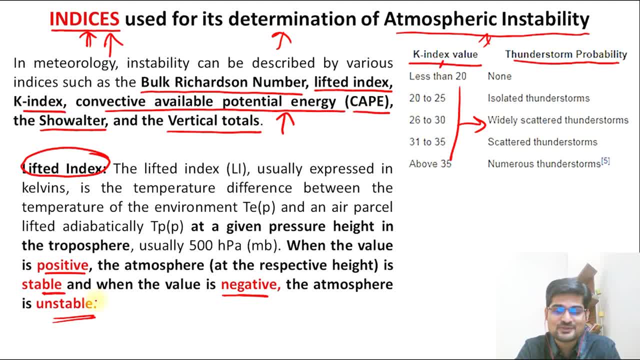 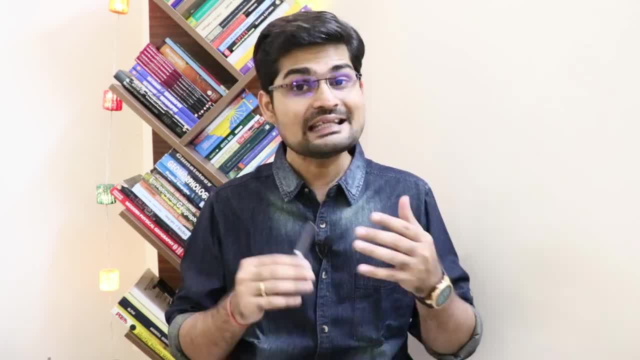 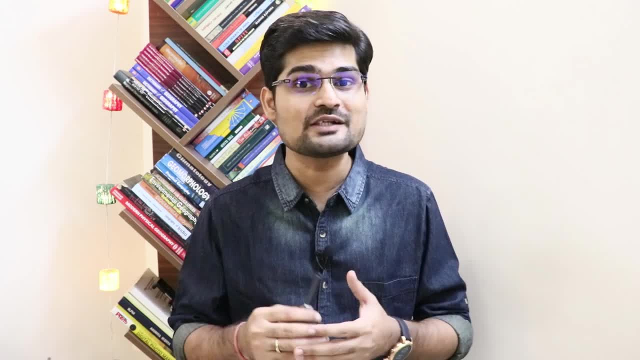 atmospheric stability and instability conditions. So now, when we have discussed the nuances and details of this atmospheric stability and instability, in the lectures to come we are going to learn about the winds of different types, that is, planetary winds, seasonal winds, local winds. So stay tuned, stay safe and keep watching.